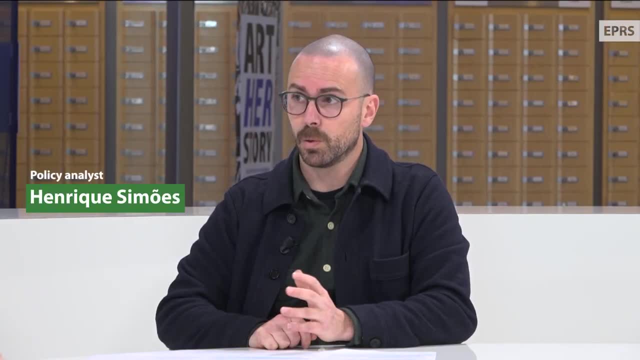 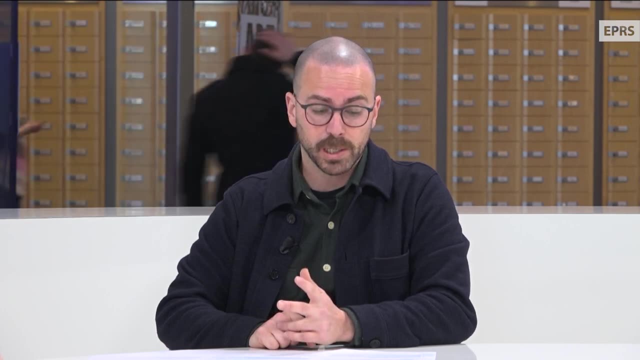 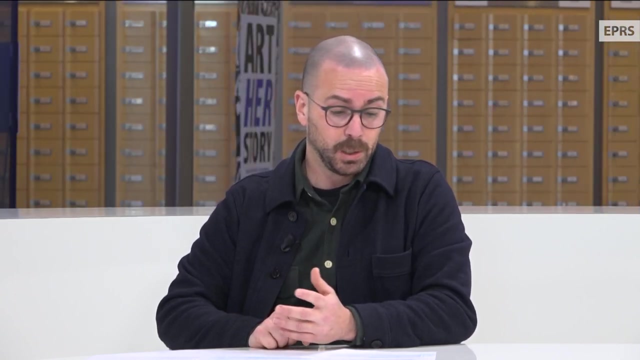 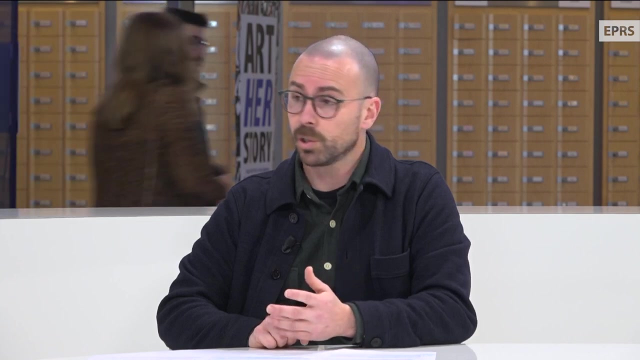 is the process of adjusting to actual or expected climate and its effects. It is important to define three important concepts in order to act on climate change adaptation, The first one being vulnerability, which is how likely are you to be adversely affected. The next one is risk, which is the potential of negative consequences. 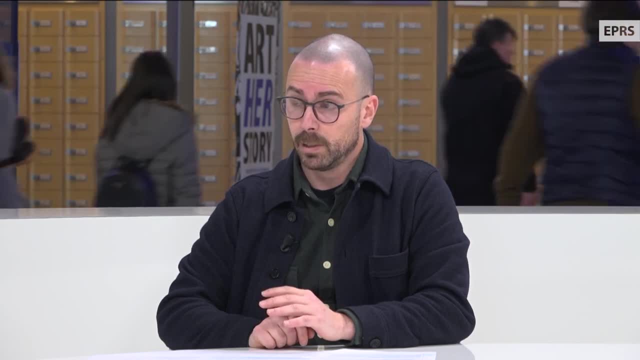 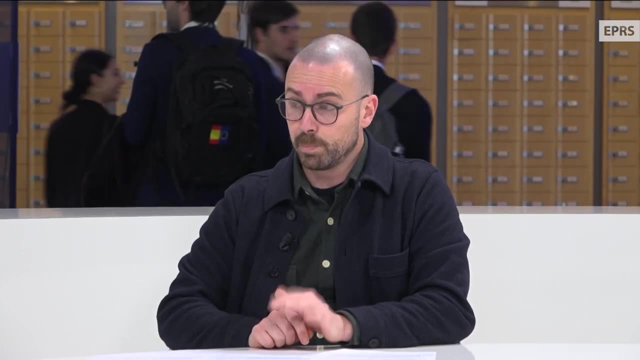 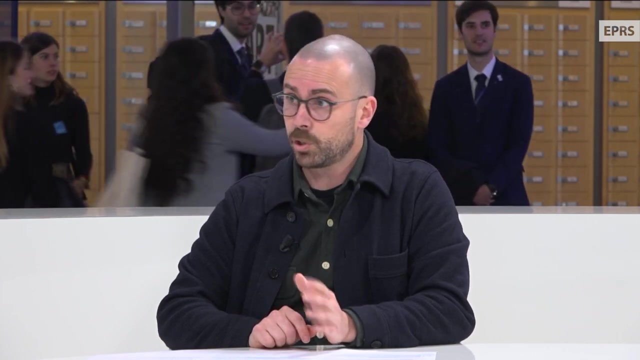 when something of value is at stake. And the final one is impact, which is the consequences of the risk in the system. It is important also to highlight that there are limits to adaptation, So in some cases there is no chance of adaptation, like, for example, island states where there's no chance for population. 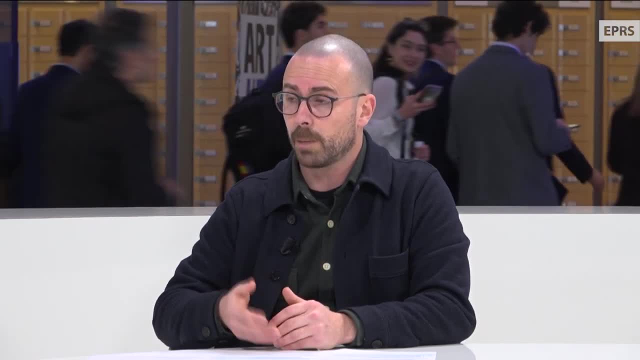 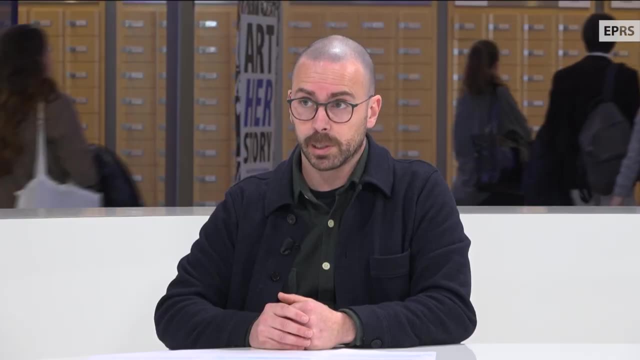 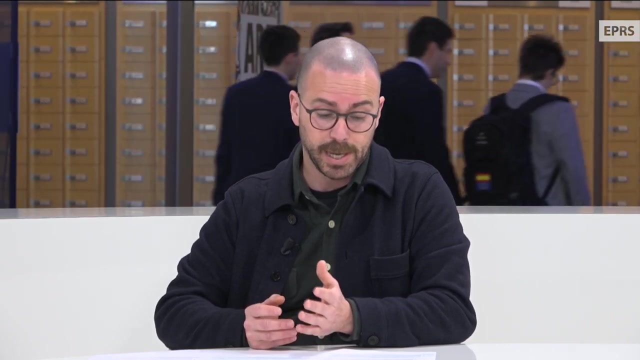 relocation or in other cases where the option to adapt it's still not available And is climate change a priority globally? Currently, the parties to the United Nations Framework Convention on Climate Change. they already have plans, strategies, laws and policies that are getting better and more inclusive. 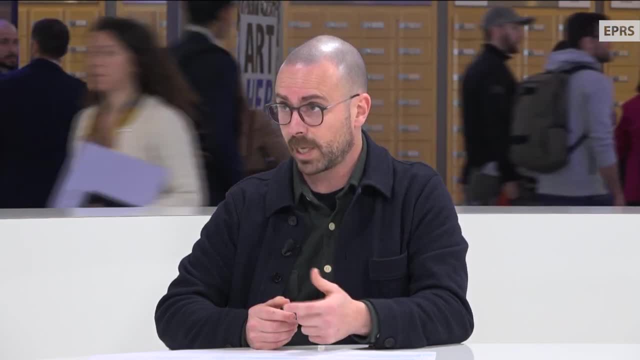 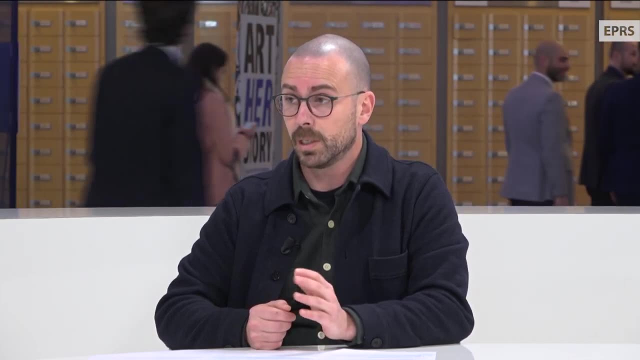 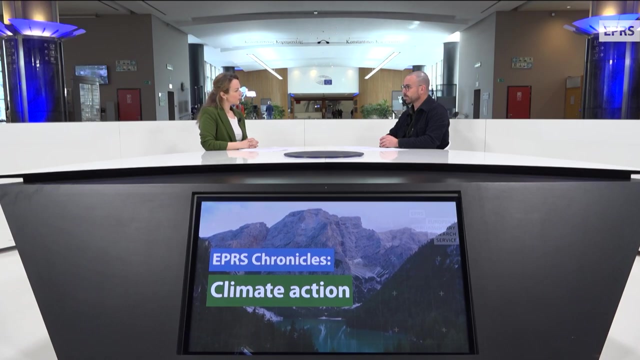 But they're still lacking funding in order to take the next step, that is, to pass on to action. The international funding that is directed towards developing countries is also identified as being five to ten times lower than it should be by now, So would you say that we are falling short? 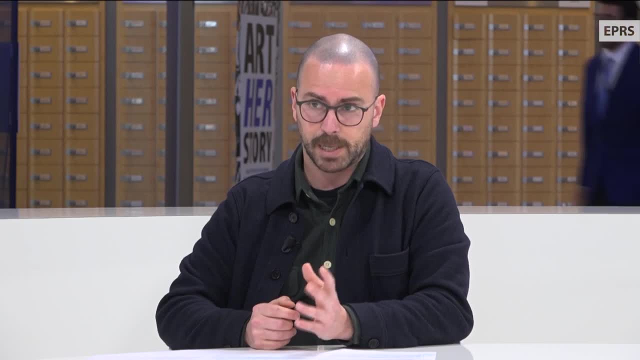 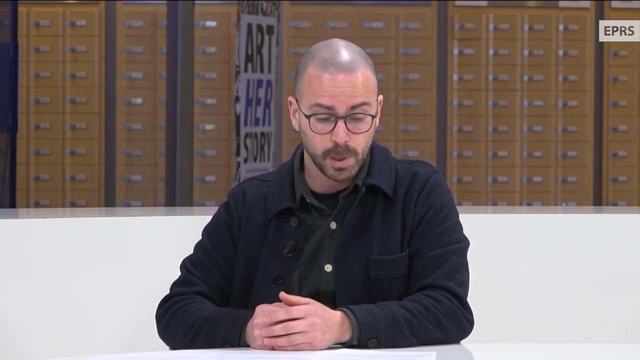 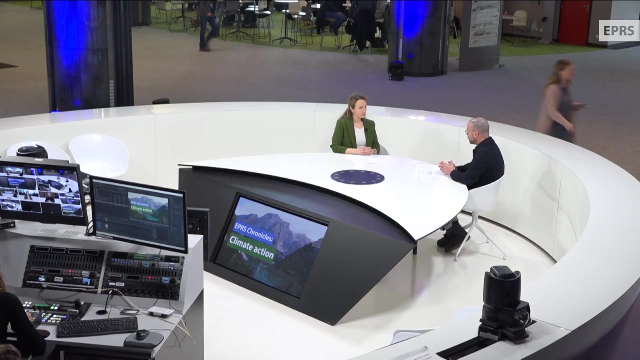 Well, I wouldn't say that, because implementation of adaptation actions are increasing, including the ones that involve nature based solutions. it's not keeping up with climate impacts and therefore we need a strong political will in order to increase adaptation investments and outcomes. In a nutshell, global efforts are being made. 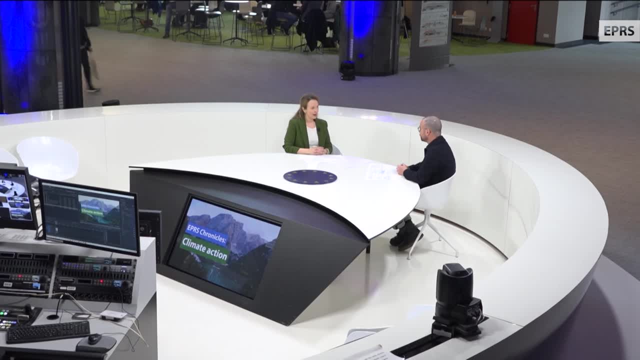 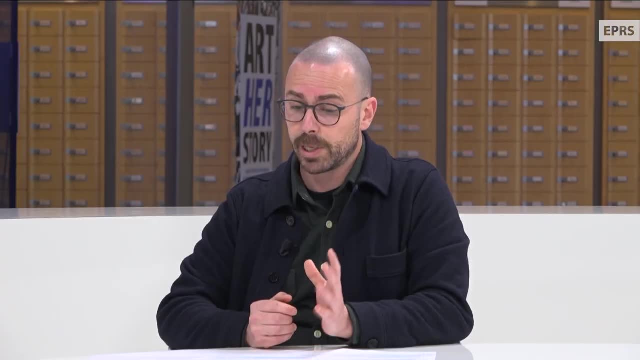 but the funding is still lagging behind. And what about nature-based solutions? Can you tell us what their role is in climate change adaptation? Well, nature-based solutions: they encompass a range of ecosystem-based approaches that aim to increase the resilience to climate change. 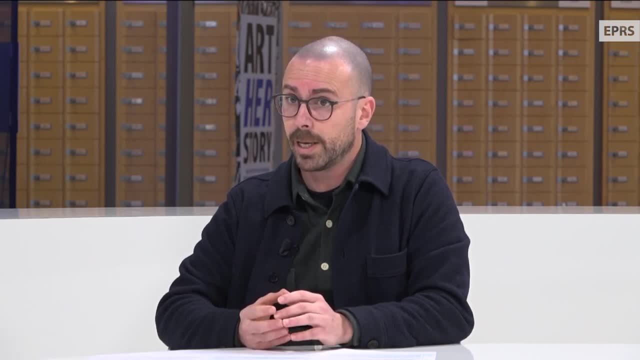 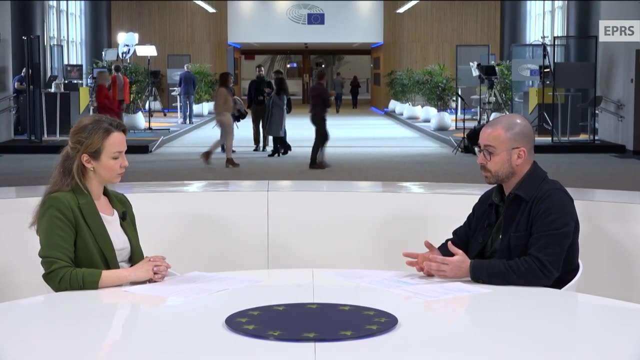 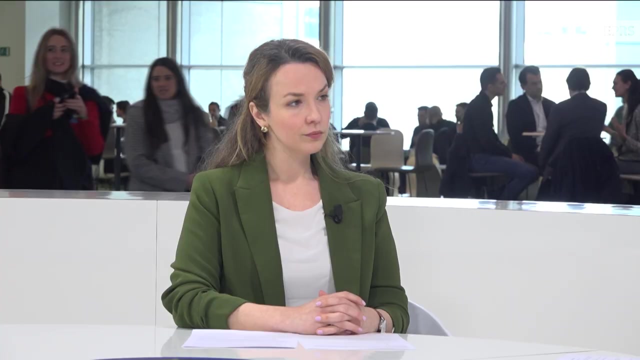 Those are typically stakeholder-driven and they are tailor-made for a specific region or local. They can deliver services such as erosion control, drought or flood prevention. The examples of nature-based solutions typically include coastal zone protection, wetland restoration and agroforestry, amongst others. 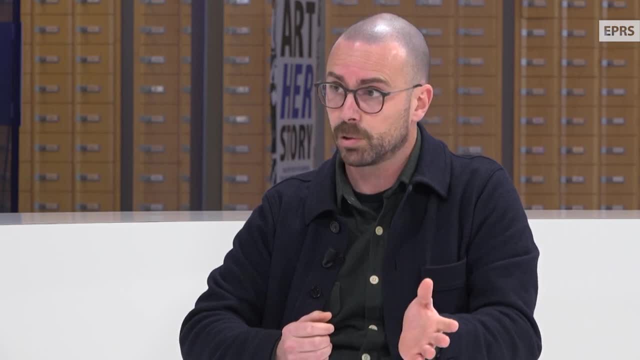 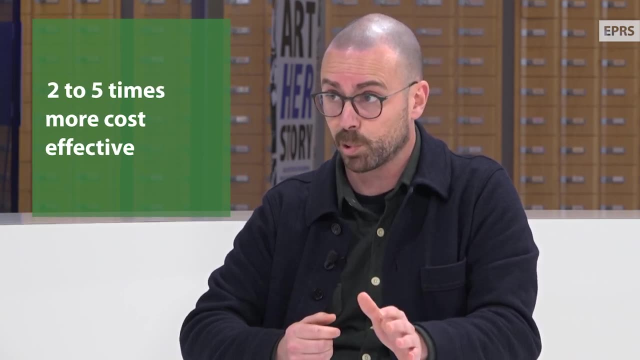 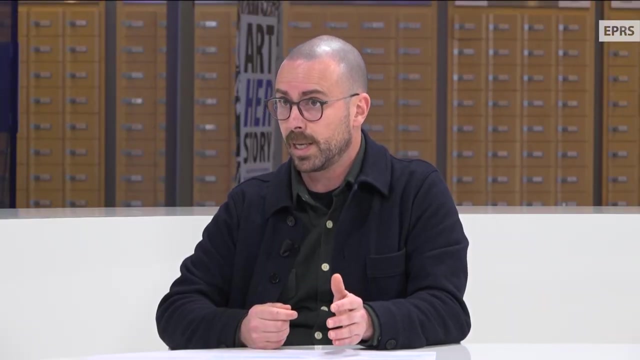 And it's curious enough that some natural coastal defense projects they have been found to be between two to five times more cost-effective than engineering projects. Nevertheless, there are still knowledge gaps to be filled in order to fully roll out these solutions as a valid climate change adaptation action. 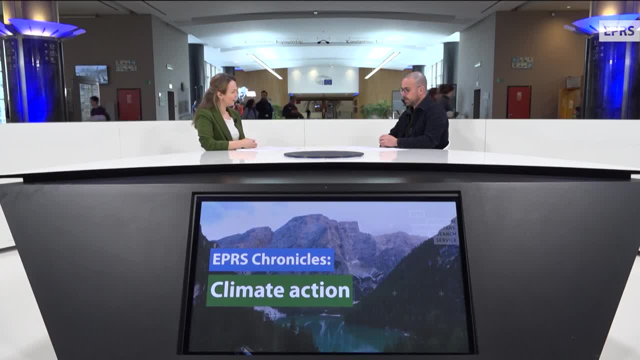 Well, what kind of knowledge gaps are we talking about? Can we fill them? Well, knowledge is vital to make the correct choices, And when we're talking about climate change adaptation, which needs effective actions, we feel that there's the need to gather more. 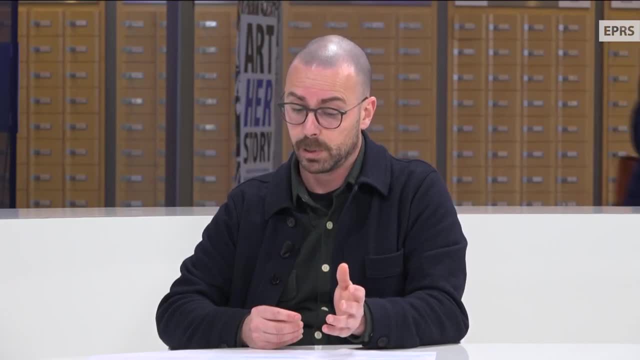 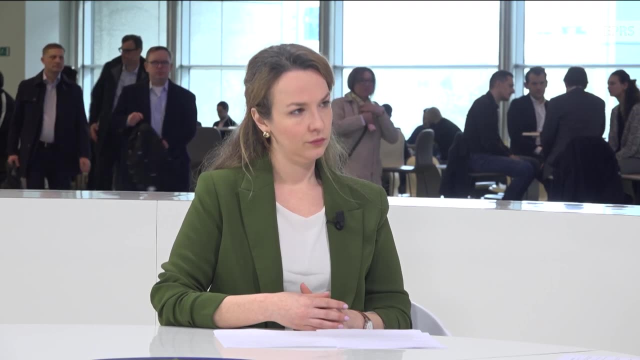 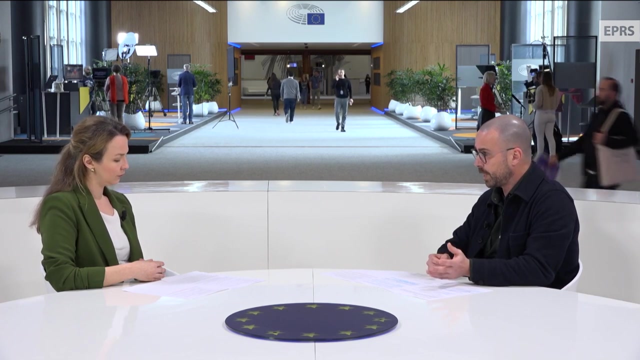 and better information, especially on economic losses. Currently, there are a number of sources that are available to the public. They are open source. Some of them are tailor-made for local authorities to go and find information. Amongst these, we have the Climate Adapt platform. 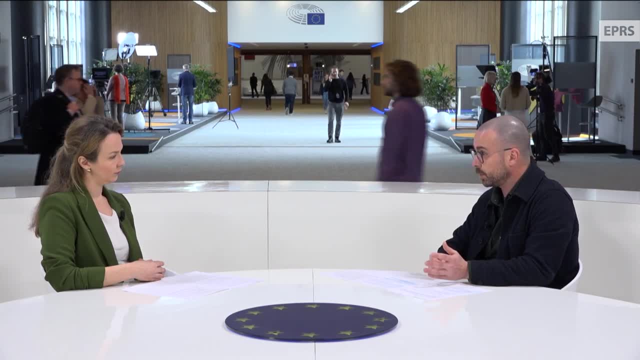 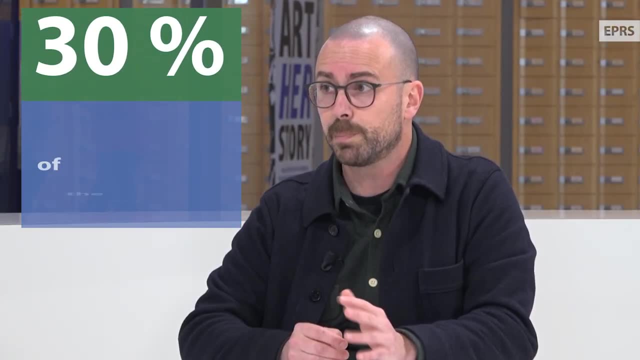 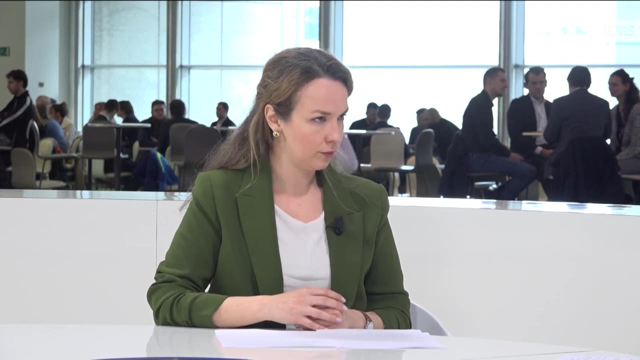 or the Covenant of Mayors on Climate Change and Energy, which currently count with a little over 11,000 signatories and represent roughly 30% of the European population. And you mentioned open source: What would be accessible at a local or regional level? 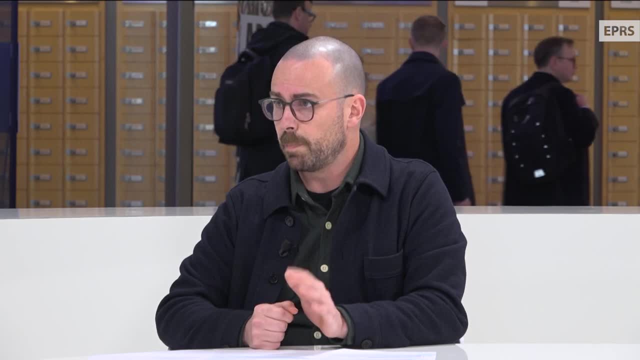 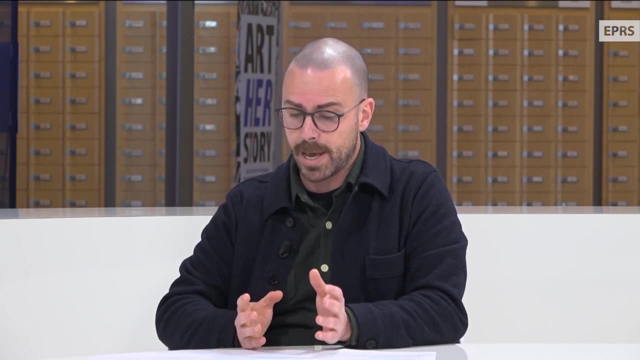 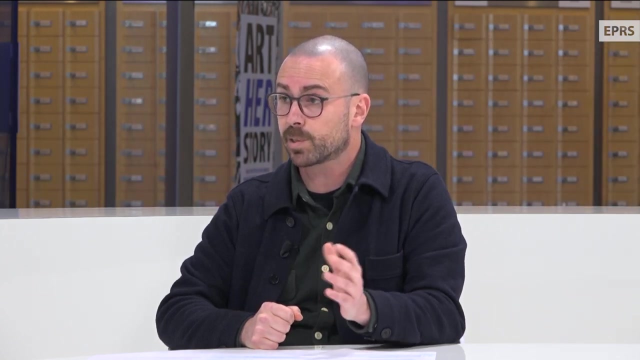 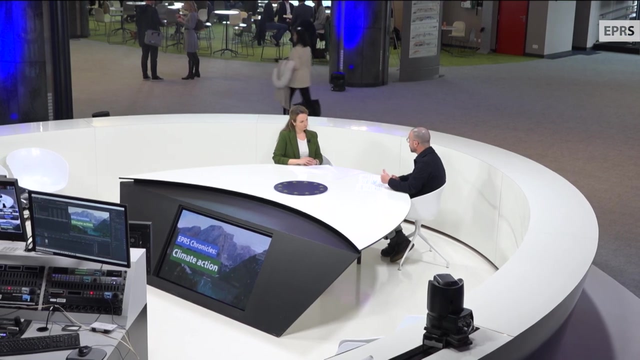 The local or regional level has been identified as being one of the major key stakeholders within the adaptation processes And both within the Covenant of Mayors. there are a multitude of tools and and services provided, like in project matchmaking, But in terms of nature-based solutions, it also exists. 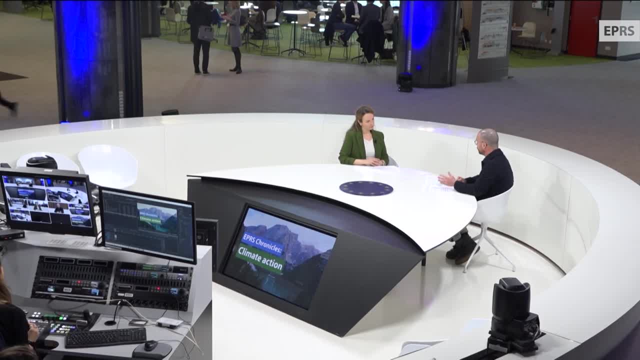 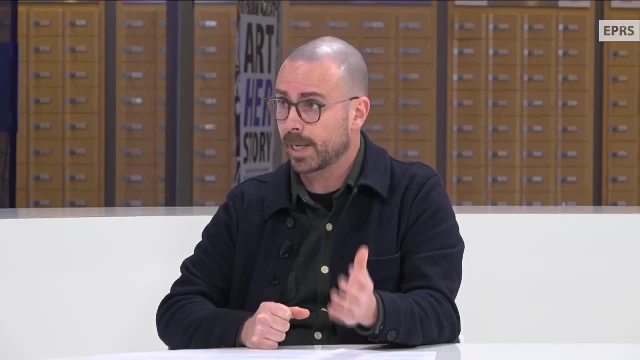 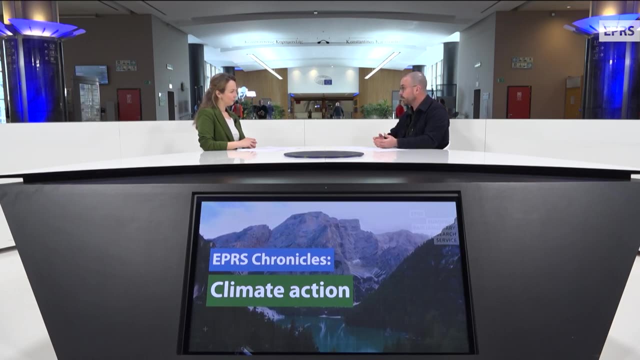 There are numerous open source platforms available to the local and regional level. I would just like to highlight one that was able to develop a handbook and an appendix of methods that local and regional authorities and everyone in general can make use in order to identify the best nature-based solution. 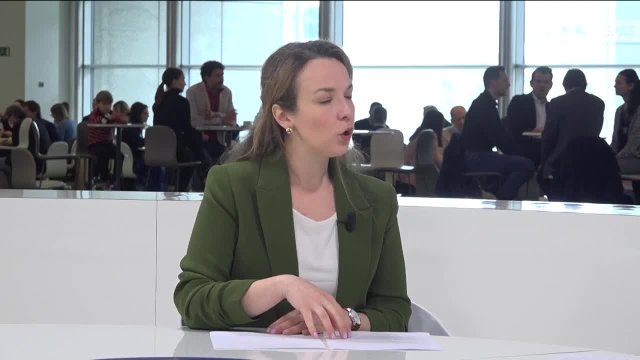 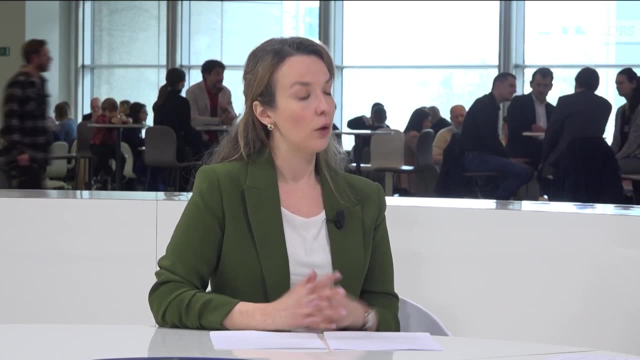 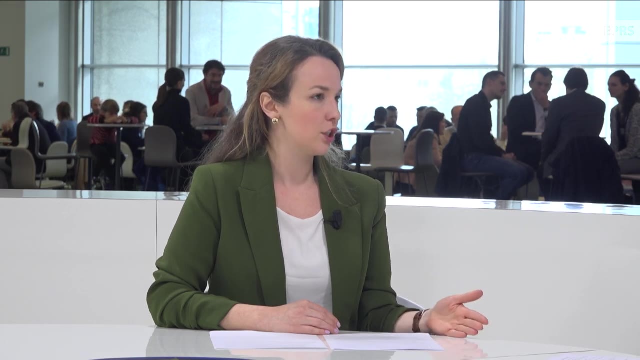 for their intentions. I'd like to briefly go back to something we spoke about in episode two in more detail. We mentioned mitigation of climate change and what the EU is doing in order to mitigate its effects. Do we see a link, a relationship between climate change mitigation? 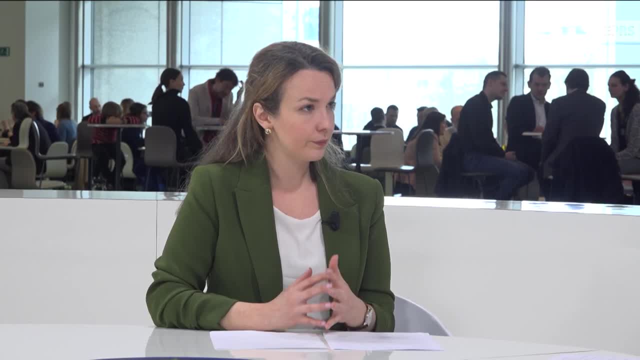 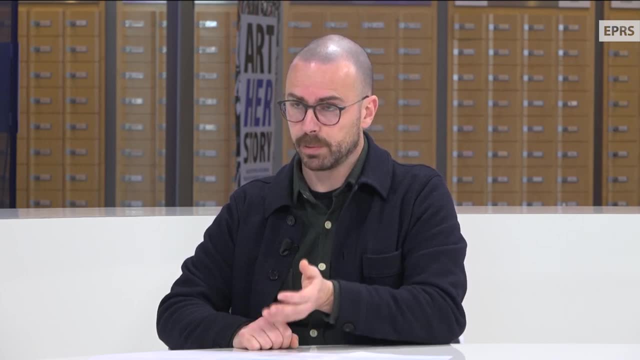 and climate change adaptation. Could they work jointly? Well, that's a good question, And there are potential benefits in having them both work together. As we know, mitigation actions take a long time to effect rising temperatures. Therefore, adaptation to current change is needed. 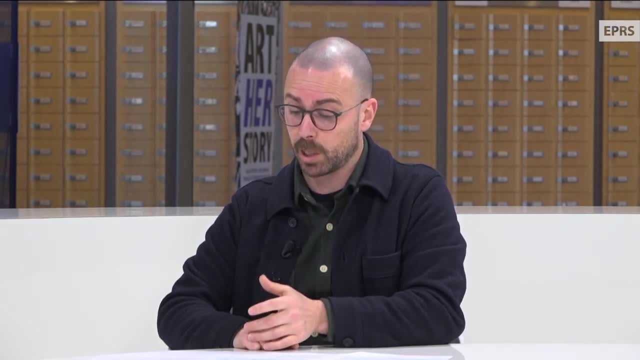 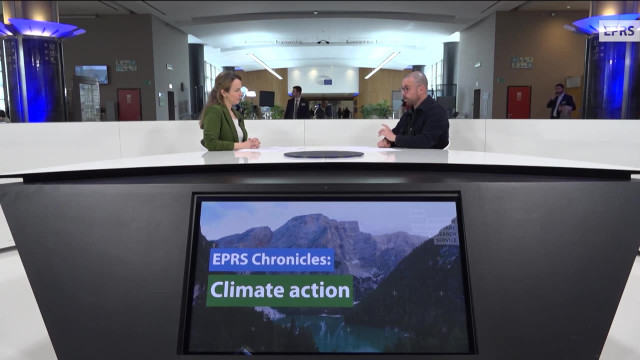 As both mitigation and adaptation address the same cause of impact, they need to work in an integrated manner to successfully achieve their respective aims. There are opportunities to be taken when integrating mitigation and adaptation aspects at the same time in different stages, being at the planning stage. 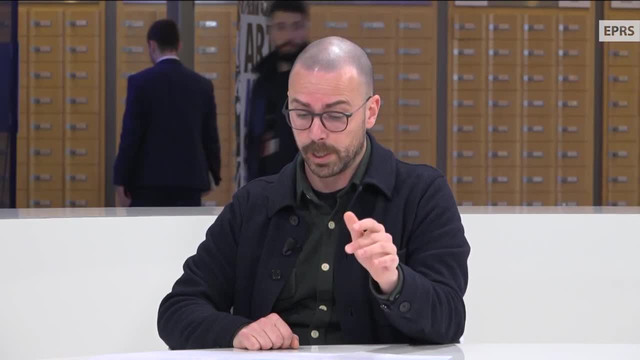 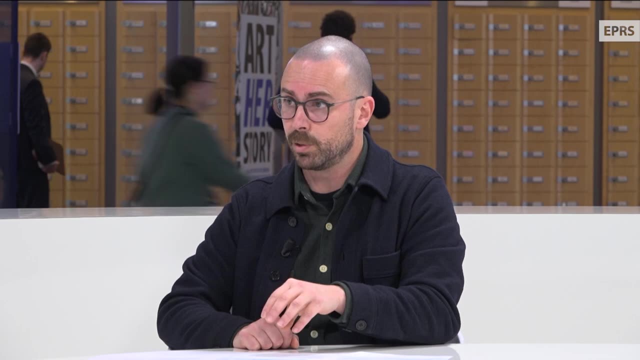 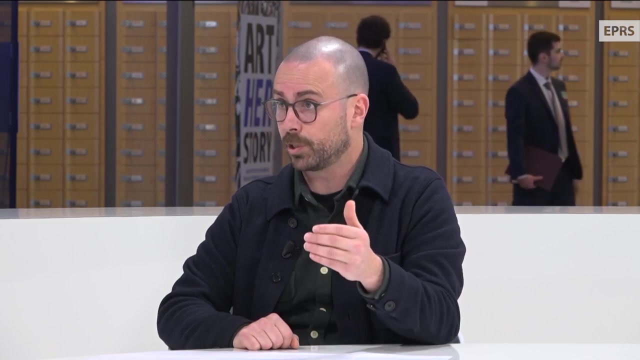 stage, in the investment stage or the finance stage. One example of this could be an adaptation option that chooses to increase the use of air conditioning units, which would then mean that we would have an increased consumption of energy. That trade-off can be minimized if we mitigate that consumption of 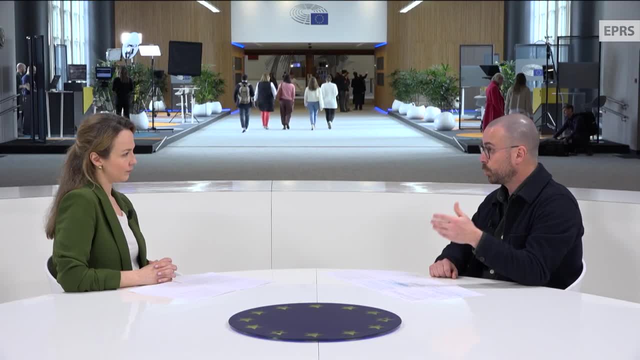 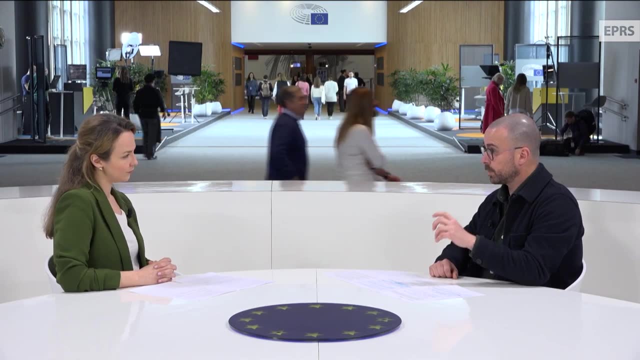 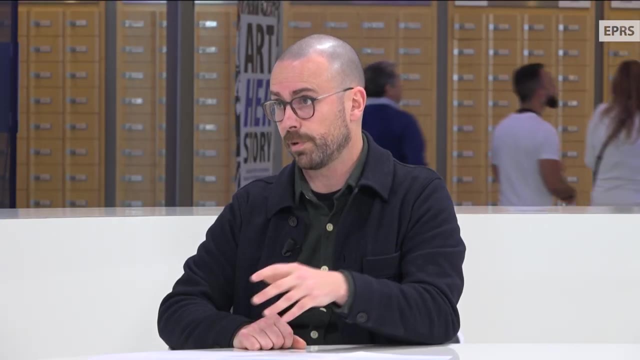 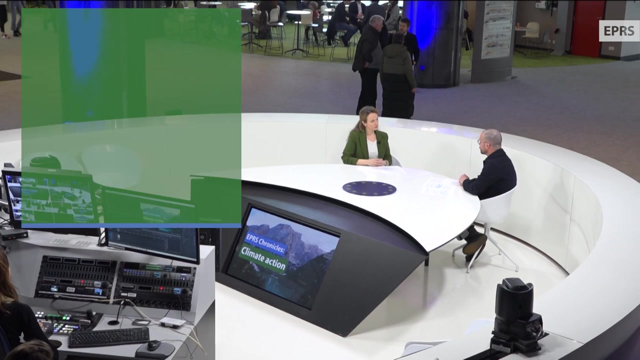 energy by introducing a renewable energy source to power those air conditioning units. But nevertheless, funding that addresses simultaneously adaptation and mitigation actions is still very, very short. Where does the EU stand when it comes to climate change adaptation? Well, the EU launched this first strategy back. 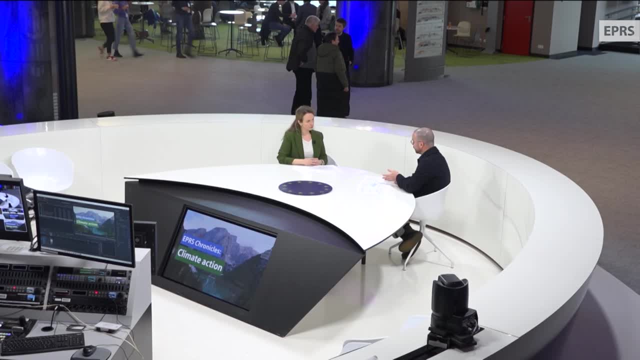 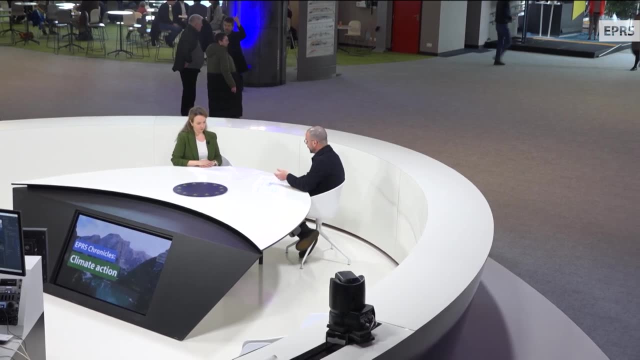 in 2013.. In 2021, it revised the strategy and, even if it did not introduce any legislative proposals, it was still very, very short. So it's still very, very short, But Lets take a closer look at the lines presented by the EU, As you can go. 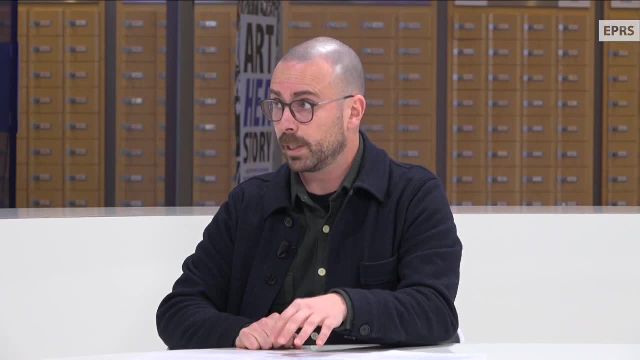 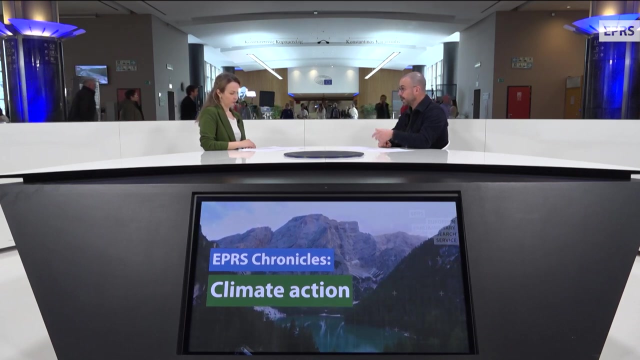 through each one, the. there is a big difference between the national framework proposed for one of the key areas. Firstly, it looks at the base sehen, the new loans and할 esem is on the growth in previous cycle. Furthermore, among the points they were the one for Olulate v OMJ- Excellent.